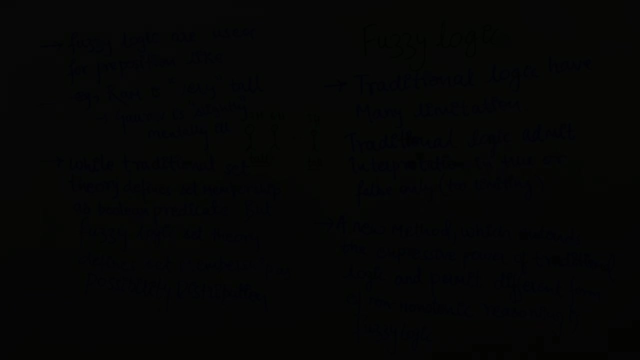 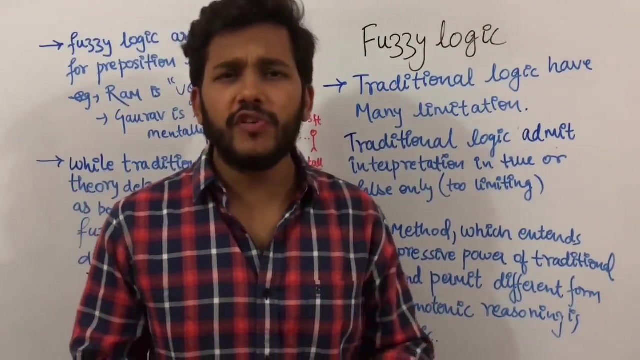 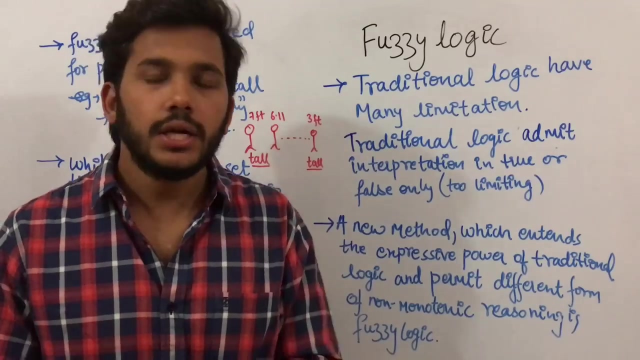 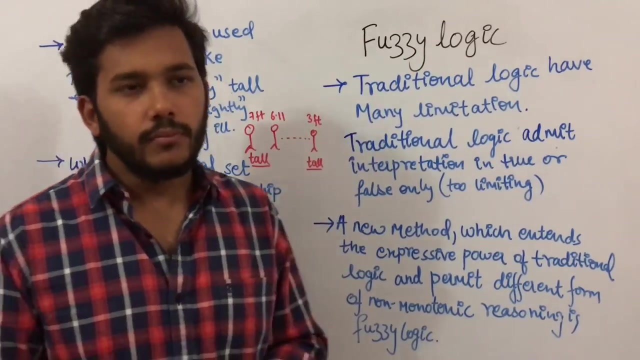 So, hi guys, in this video I am going to talk about fuzzy logic. Before we discuss about fuzzy logic, or what is fuzzy logic, let's discuss: why do we need fuzzy logic? When we were having some other traditional logics, then what was the need of the fuzzy logic In traditional logic? they were either: 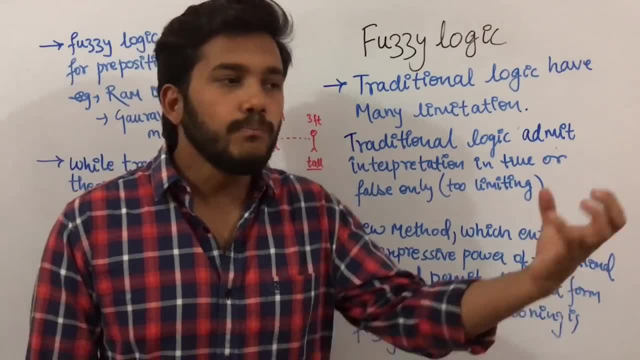 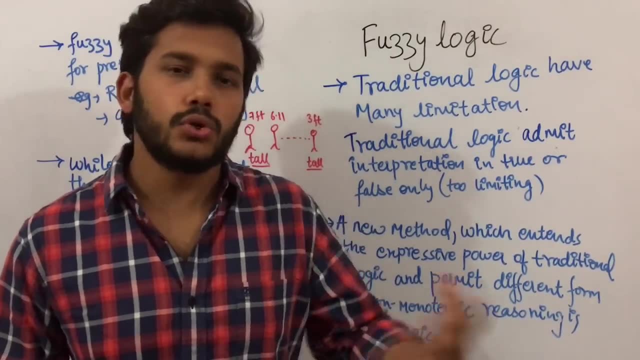 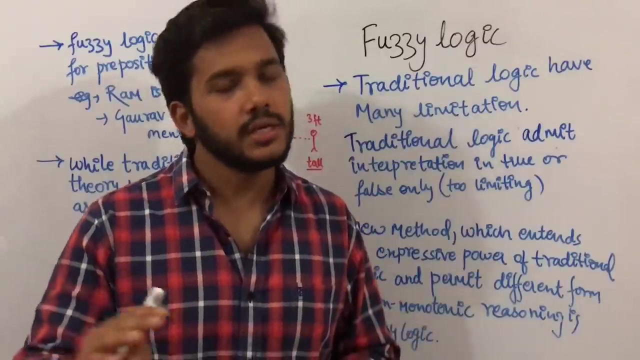 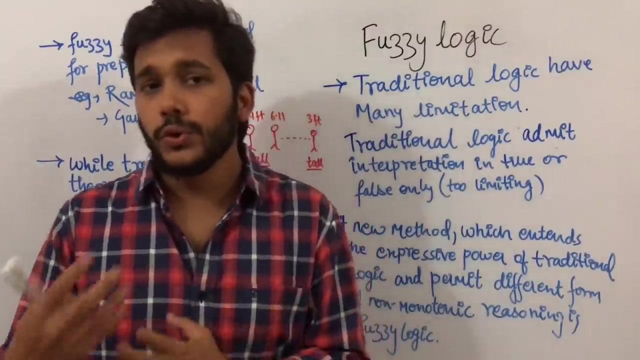 true or false. or you can say they were boolean set, that is, zero or one. In traditional logic they were either true or false. Suppose I set the parameter 7 feet height is tall and 3 feet height is small. If any person is having the height 5.6, then what you will say, it is a small or it is tall. 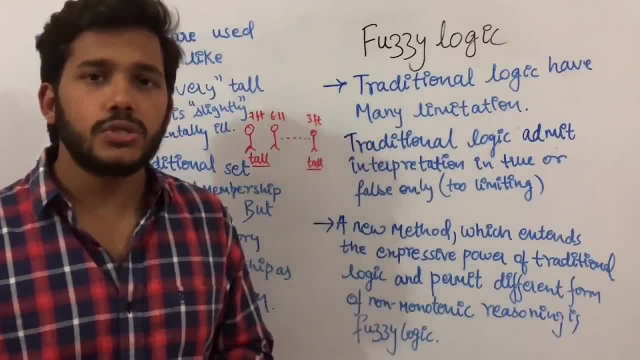 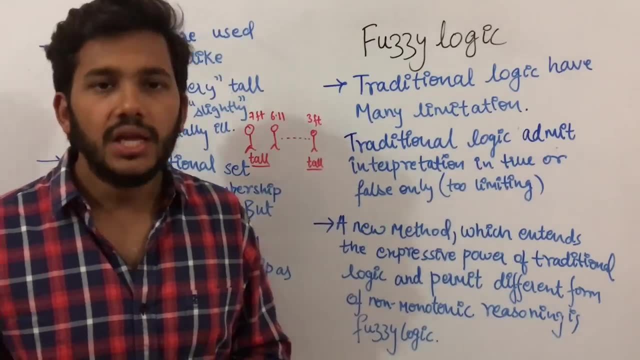 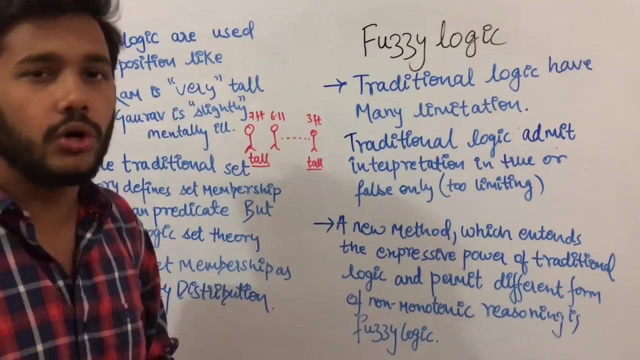 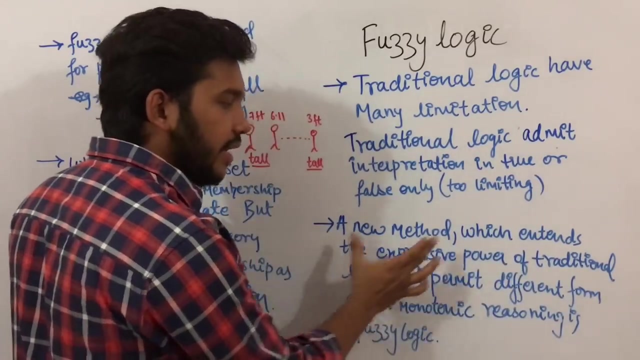 So for such type of statements or such type of prepositional statement, we need a new system that is not boolean set. This makes the fuzzy logic to come. So now let's talk about how fuzzy logic was developed. You can say: a fuzzy logic is a new method which extends the expressive power. 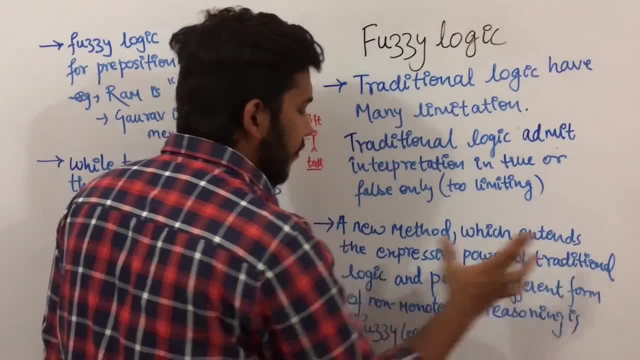 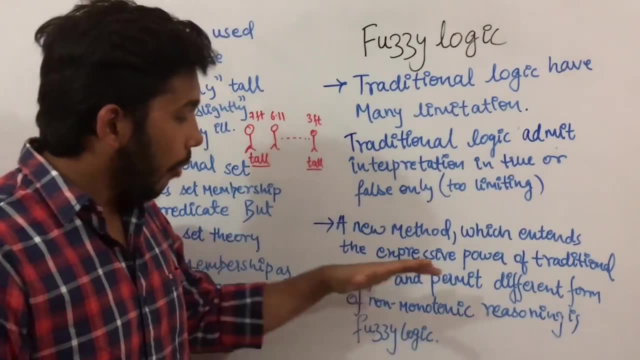 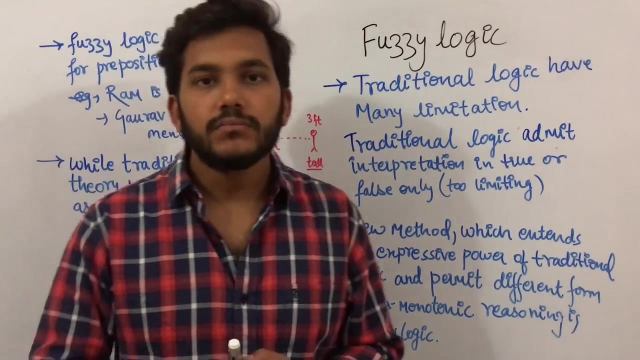 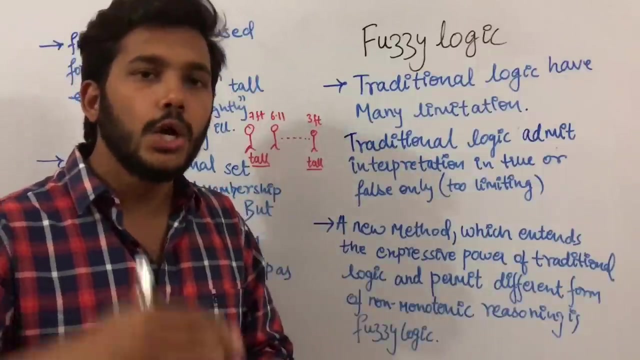 of traditional logic and permits different form of non-monotonic reasoning. Fuzzy Logic is a combination of traditional logic and non monotonic reasoning. So how itis combination? see, we are still going to solve same problem: that seven feet height was the tall and three feet high is the small. and what will be the height? 5.6. 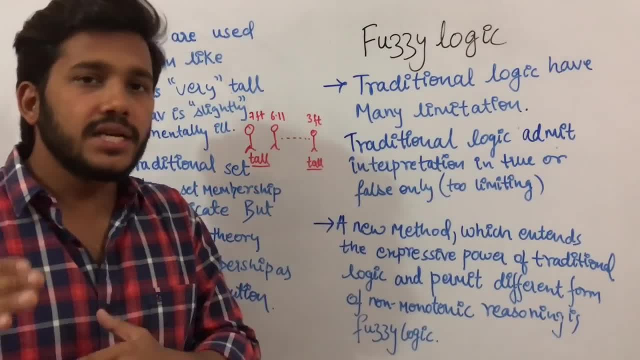 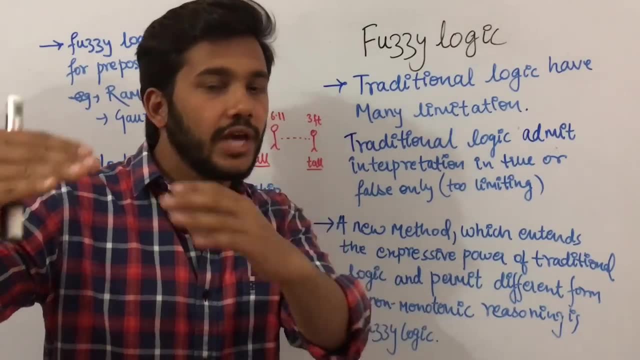 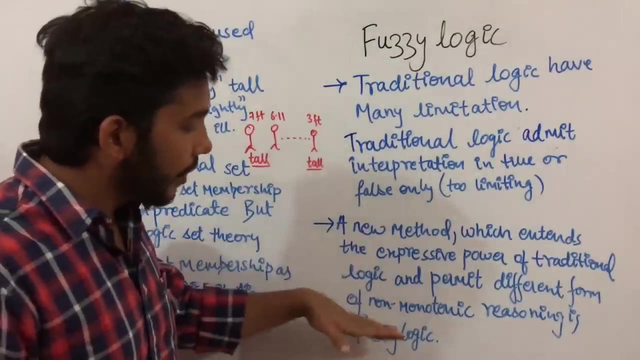 called Then for such type of parameters. just, traditional logic has a combination of mix of logic. expressive power is used means here also the tall value, 7, we are going to use, and 3 small, we are going to use. but in spite of this we are also going to use non-monotonic reasoning. we have 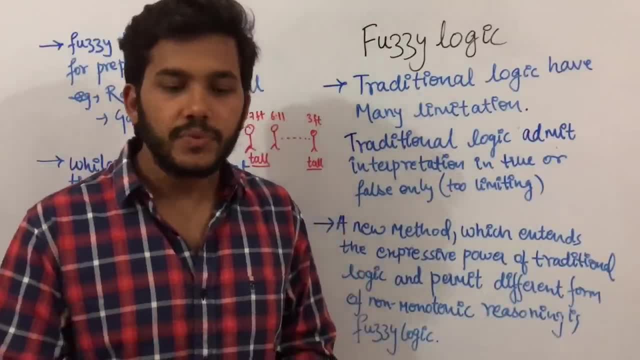 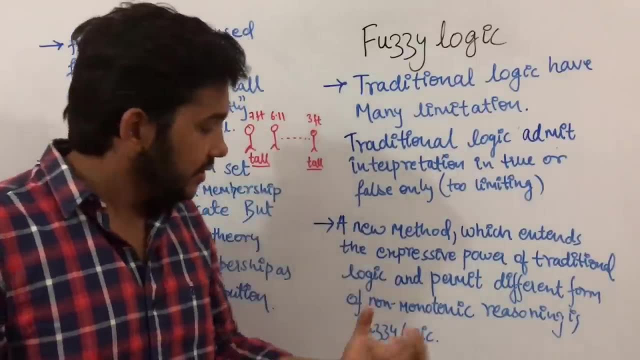 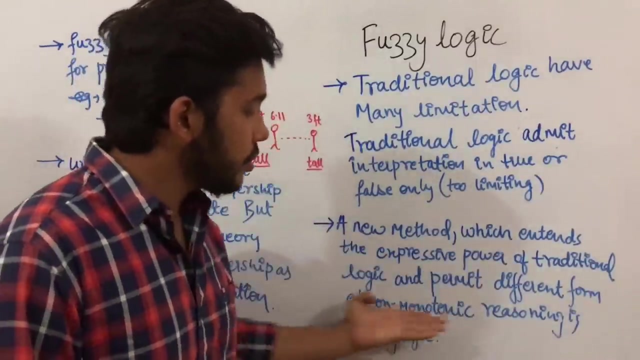 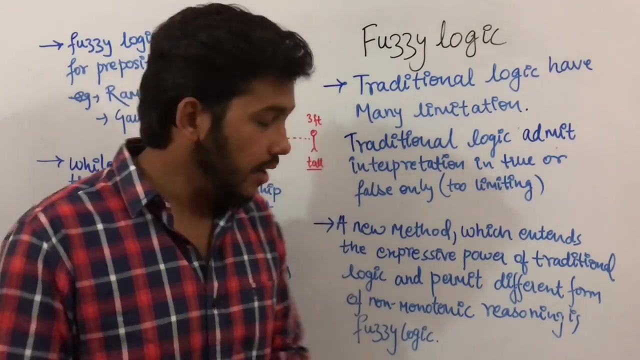 studies that non-monotonic reasoning is a reasoning. when we can reason with incomplete information or when a new data is added, then whatever our previous conclusion was, that conclusion is going to change. so this was non-monotonic reasoning. so now if i say 3 feet height is small, then i can say: 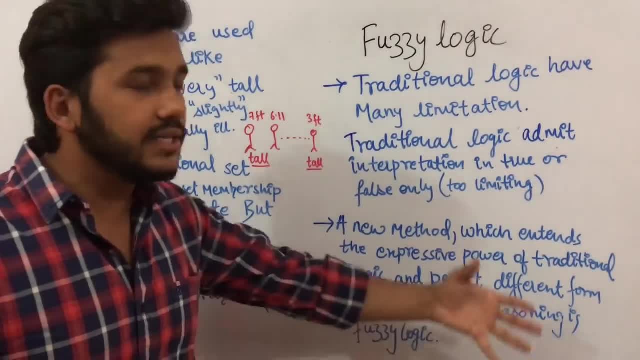 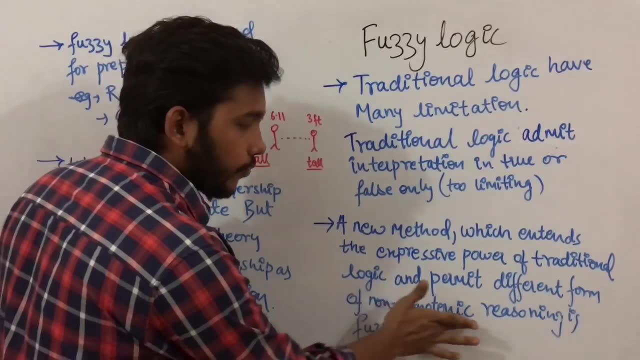 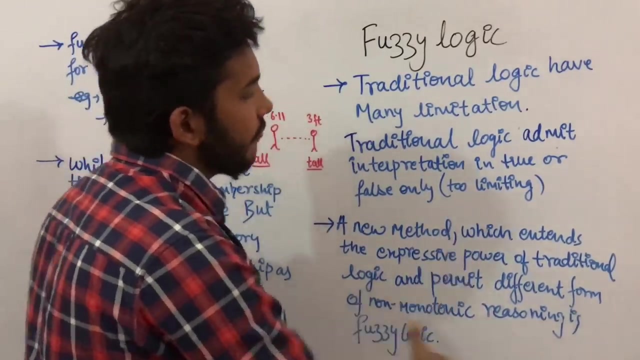 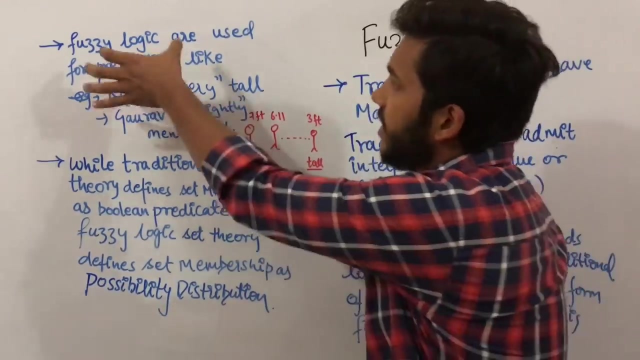 with non-monotonic height 5.6 is greater than 3, then 5.6 height is not small. so with the help of non-monotonic reasoning, reasoning and expressive power of traditional logic, we develop the fuzzy logic. now let's talk when this fuzzy logics are used. fuzzy logics are used for prepositional lights. ram is very tall. 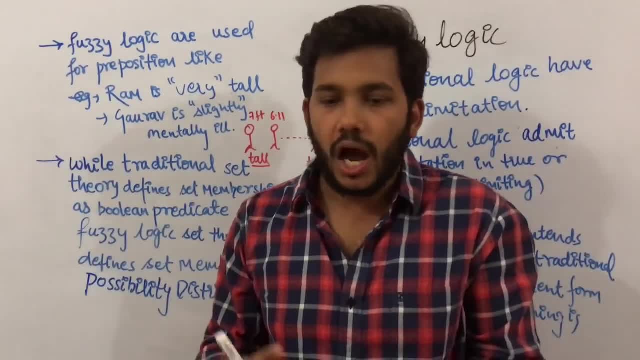 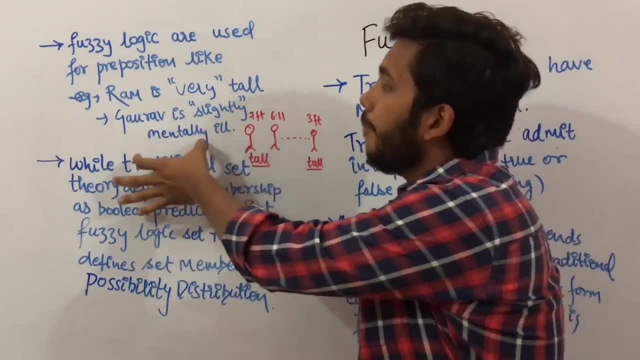 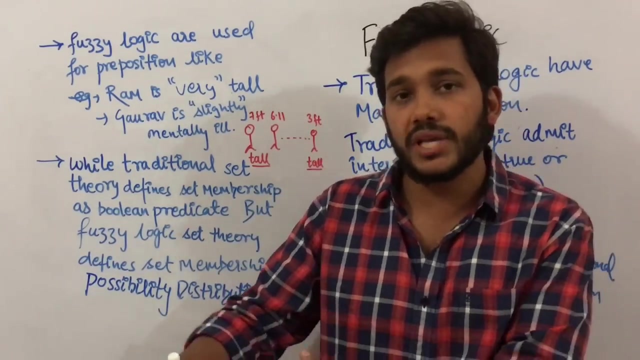 we talk about height, ram is very tall. we don't how we can compare, like if you say very tall or you, if you say gaurav is slightly mentally ill, means he is mentally ill, but i don't know how much he is mentally. it might be case if we are using 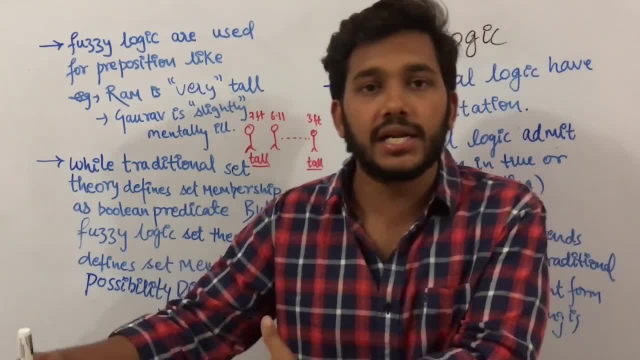 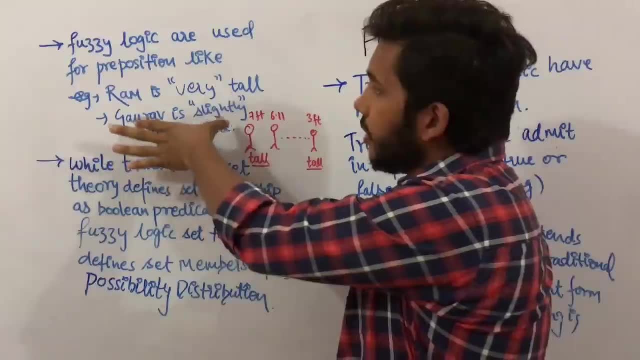 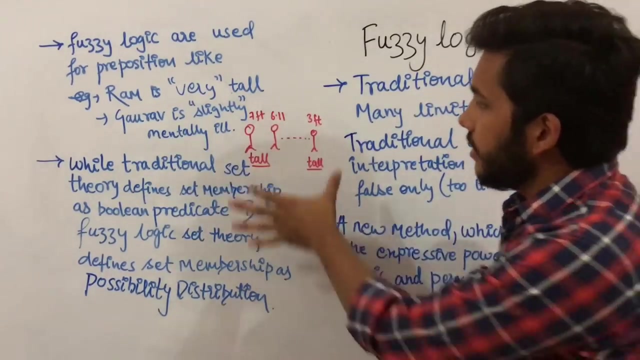 traditional logic, then we can say no, he is directly mentally or he is not mentally ill. but with fuzzy logic we can also talk about this type of prepositions: gaurav is slightly mentally ill. now let's talk an example. suppose in traditional logic we say seven feet height is very tall. 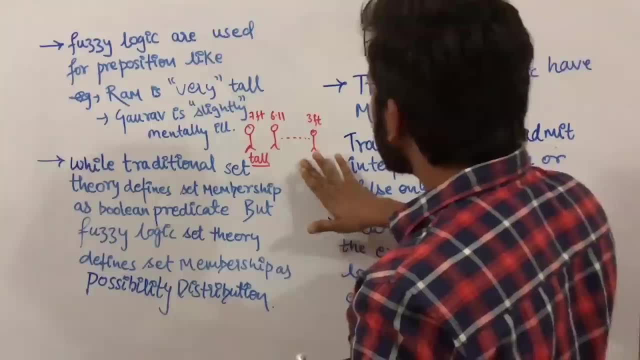 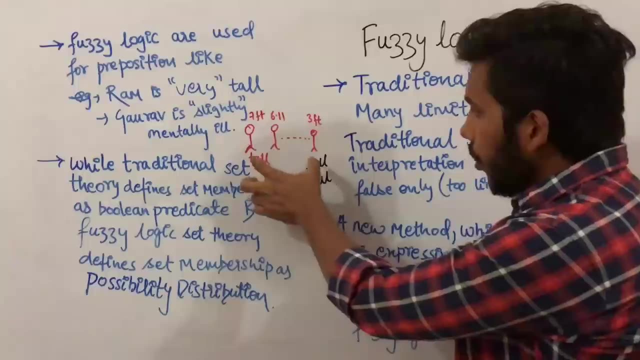 how we can say 6.5 feet height is a small height. we do here thc. we can say in: 3 feet height is tall and 4 feet height is small. source sweet, we get: 6.5 feet height is tall and three feet height is. 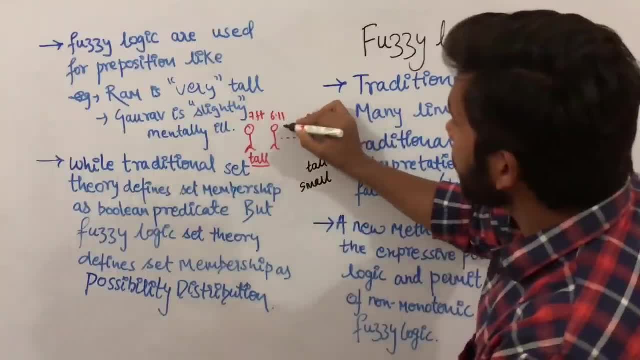 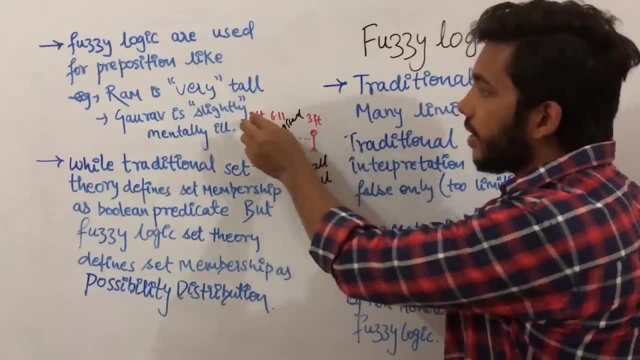 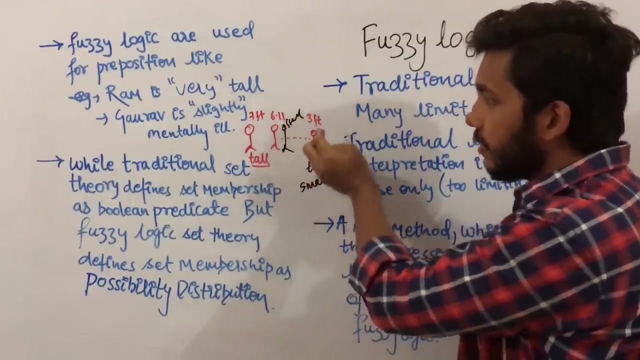 small. now with this, if we say seven feet height is short, then we can say: six point, eleven feet height is also totaled. now we can say: five foot height is also tall. why? because, slightly, if you reduce tall, 6.10 feet will be tall, 6.9, so on. so if we continue to 5 point, then we will say also that 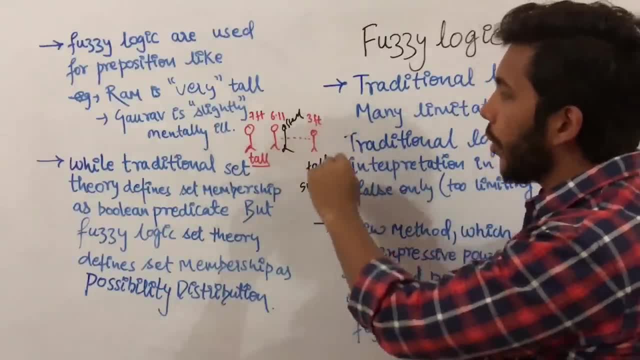 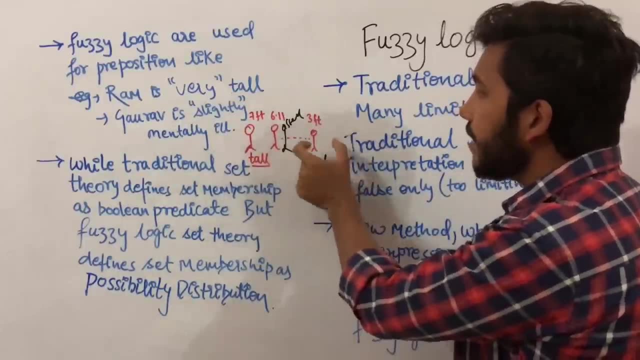 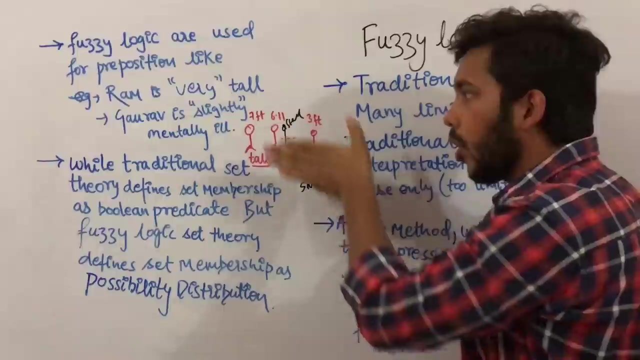 it is tall. so if we start reducing 5, then 4.9, then 3 feet. now, from this traditional logic we are going to say 3 feet height is also tall. how we say 7 feet height is tall, 6.11 feet is also tall. 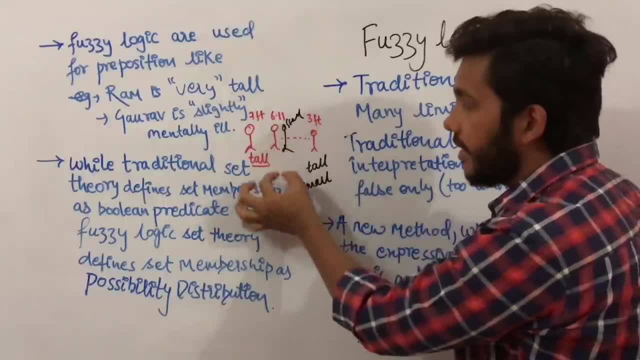 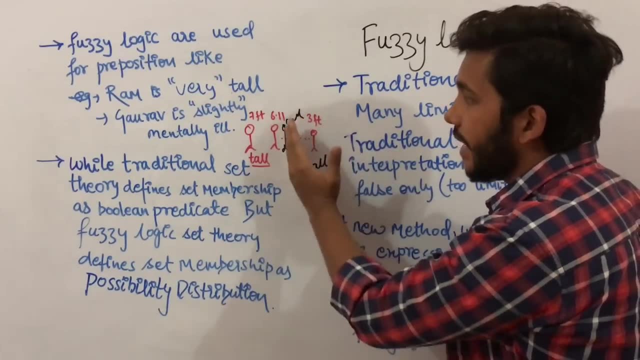 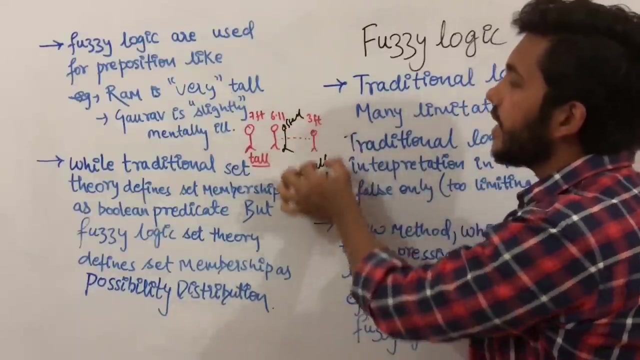 and now if we compare, if we say 6.11 is tall now in comparison of 6.11, 6.10 is also tall now in comparison of 6.10. i can compare: 6.9 is also 10, also tall and reducing. so that now, if we can also 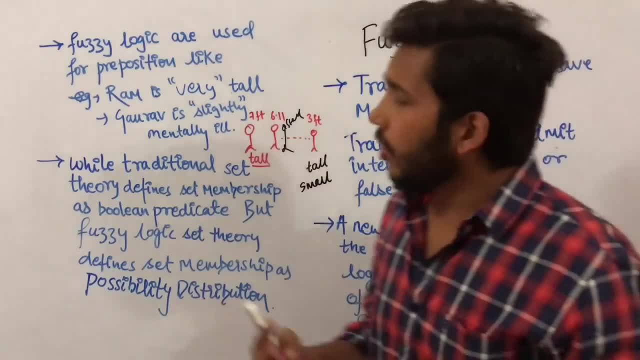 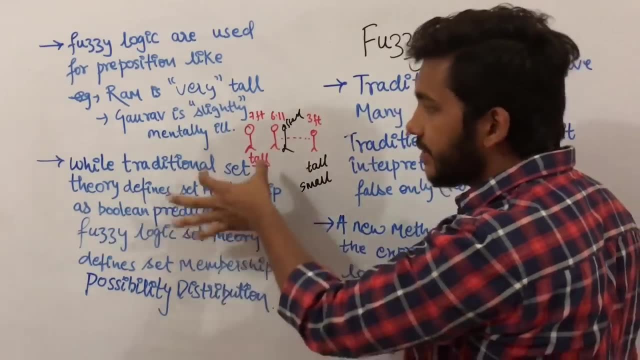 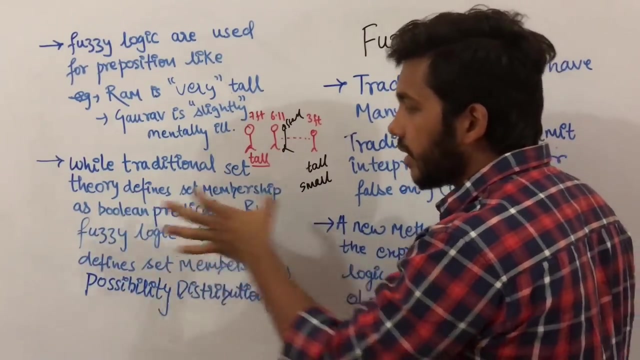 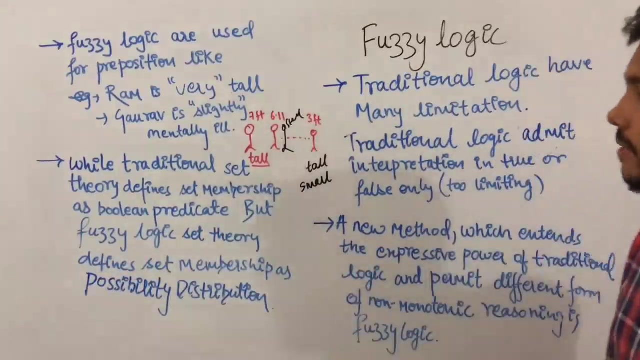 say that 3 feet height is also tall. so for this type of situation traditional logic were not good. while traditional set theory define set membership as boolean predicate but fuzzy logic, set theory- defines set membership, probability, this possibility distribution. so what, basically? this say, suppose, if we want to talk about 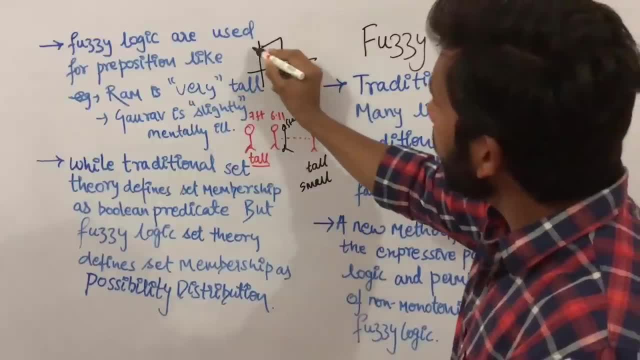 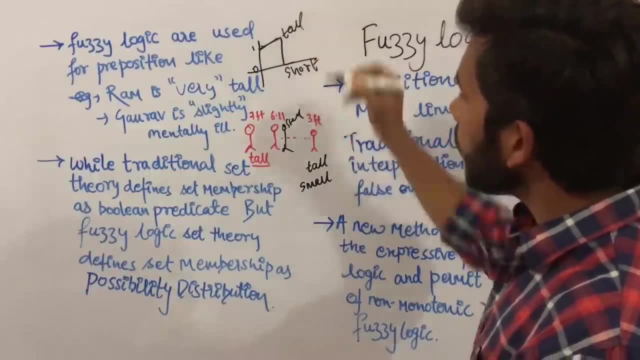 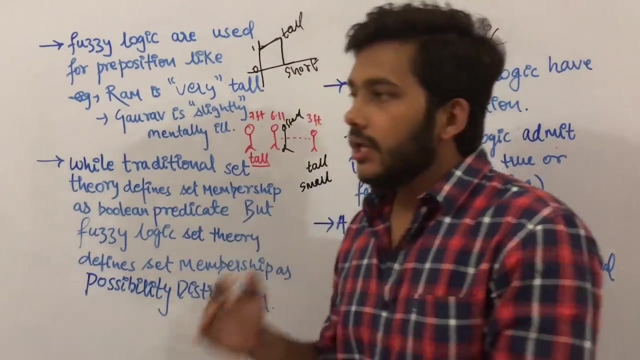 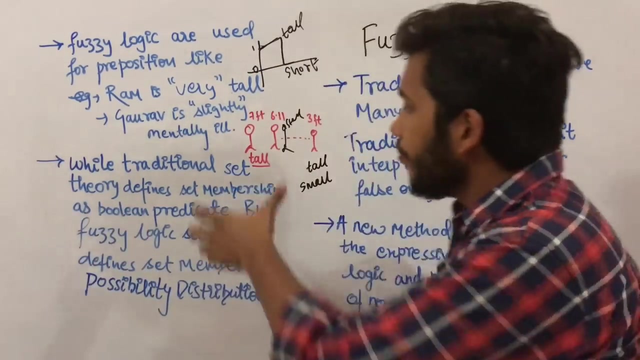 height. then in boolean we will say like this: if it is 1 or 0, this represent tall and this represent short. but fuzzy logic is possibility distribution. what are the possibility means 6.5 is slightly tall or you can say slightly smaller. so how we are going to use the fuzzy logic that i am going to to talk. 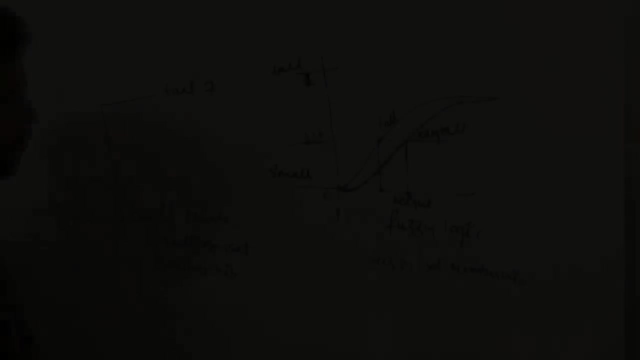 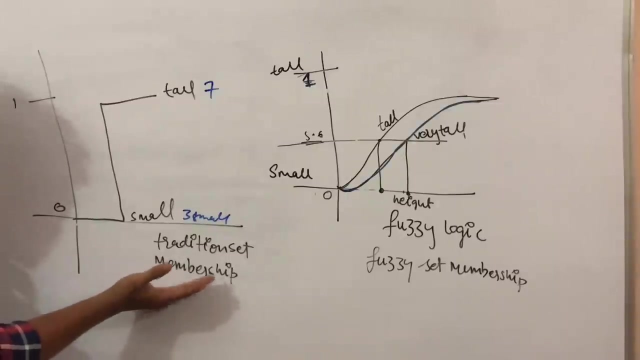 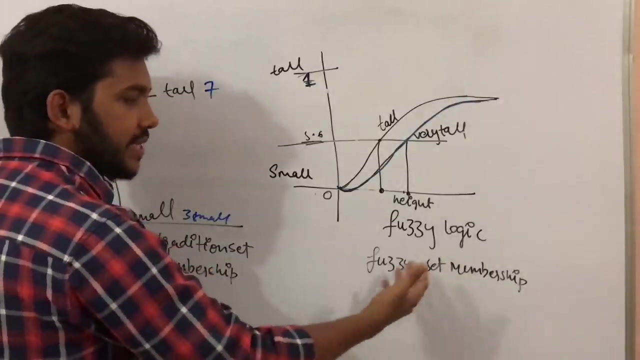 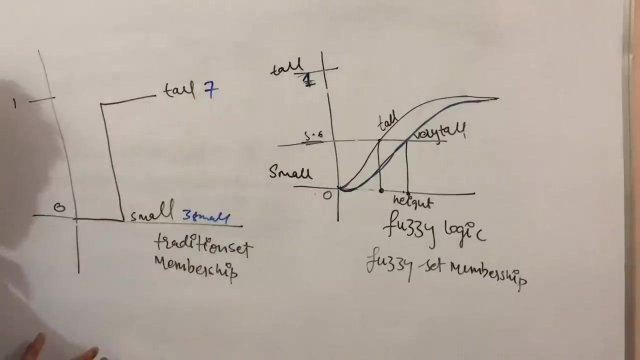 with an example. in this example, with the help of height example, i am going to talk how traditional membership was not able to express the all possibility and how fuzzy logic will express all the set membership. suppose we talk 7 feet height as tall and 3 feet height as small. 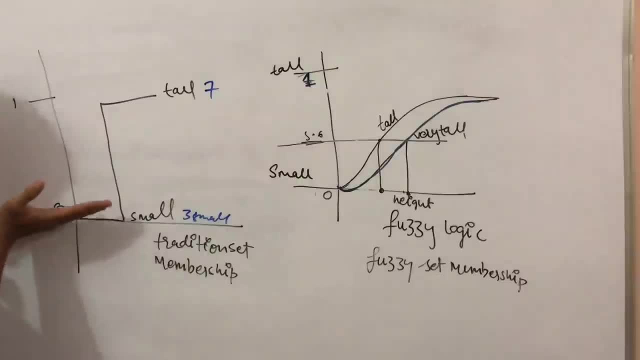 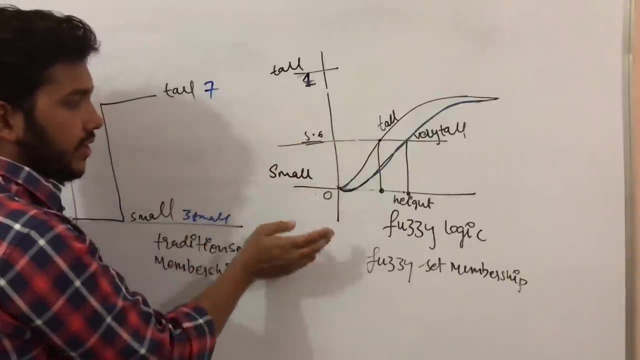 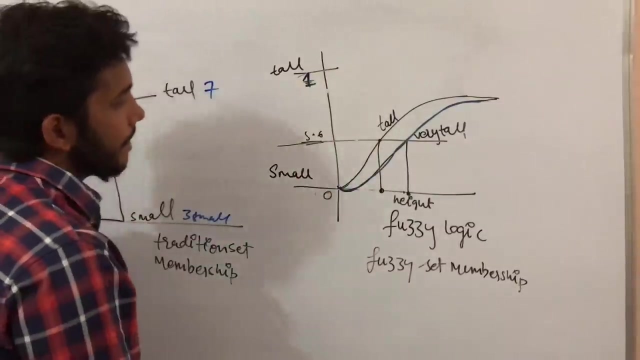 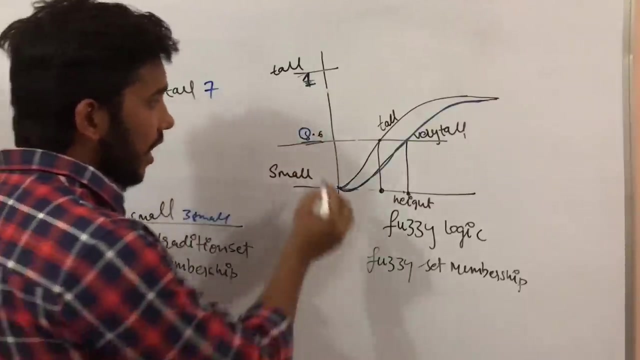 which is in the range of 0 to 1. that is our traditional logic. that is either true or false. this was there same with the fuzzy logic. we use the traditional representation, that is 0 and 1. now let's talk. there is a value that is 0.6. at this 0.6, we have two height values. 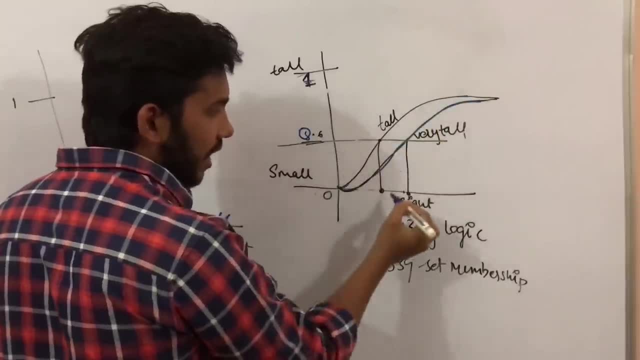 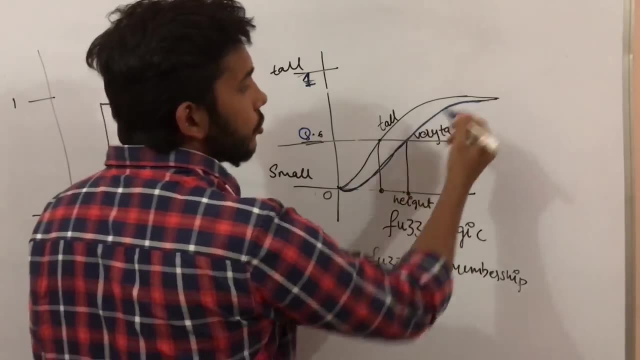 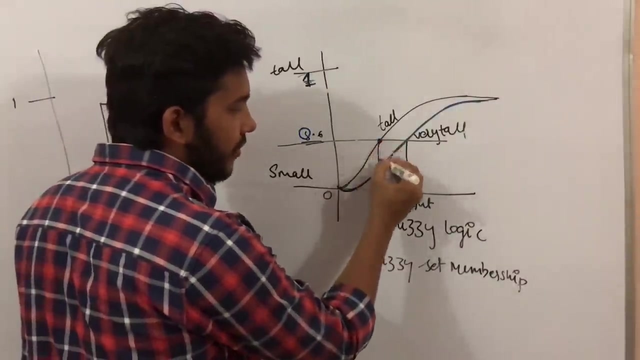 that is one that will be tall and another height value will be very tall. so in fuzzy logic set we are using this non monotonic reasoning. also, how we are using non monotonic reasoning that this particular value of the graph, if it corresponds to 4, and this corresponds to, 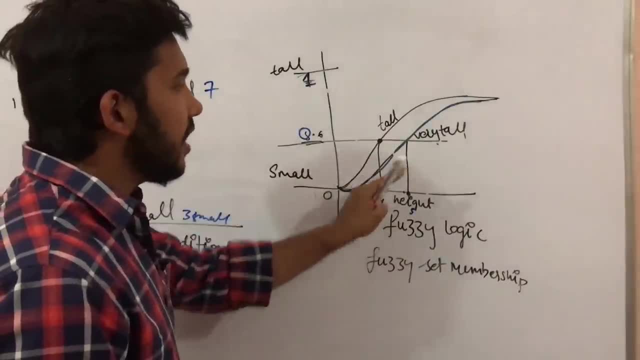 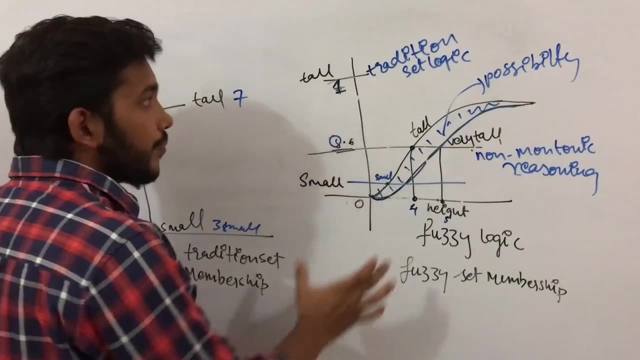 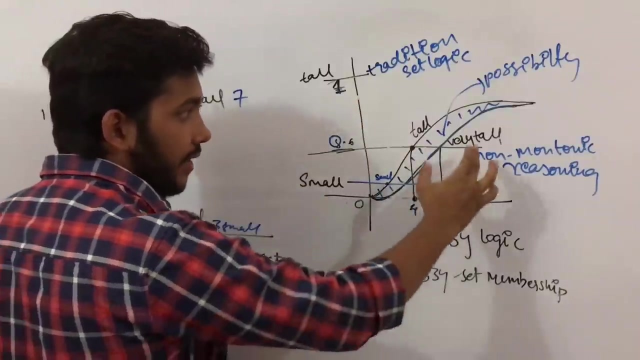 5, then you know. if this is tall, then we can say from this incomplete information that 5 will be very tall. so if we set the traditional set logic and 0 and non-monotonic reasoning in this, this is fuzzy logic set. how fuzzy. 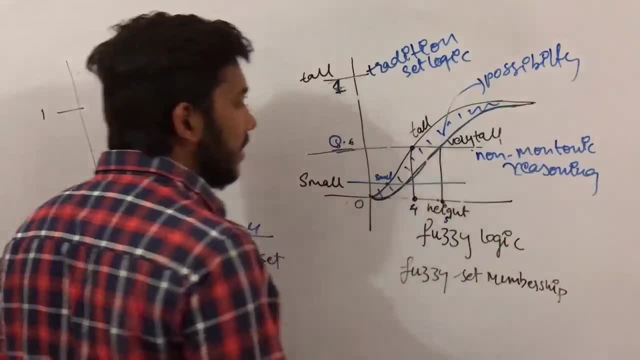 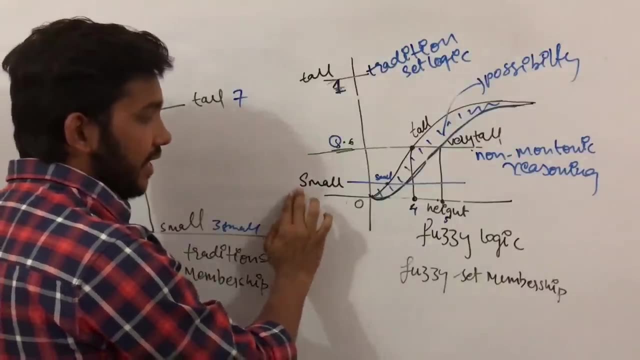 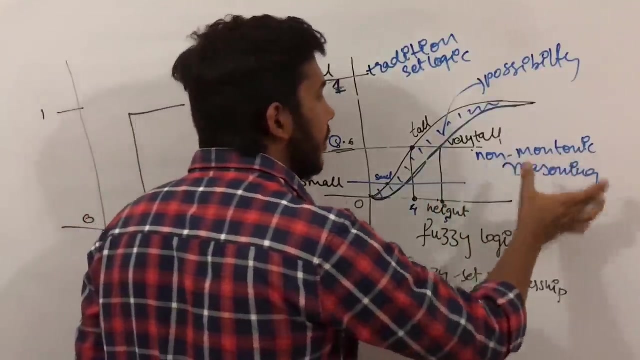 logic set is a combination of traditional set logic and non-monotonic reasoning. we have used the traditional set logic representation that we still represent 3 as a small and 7 as tall. and how we are going to use non-monotonic reasoning. see, if this is the value 0.6 and we say it as a tall, then with 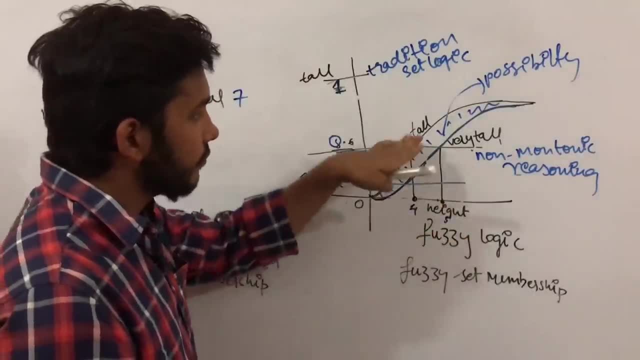 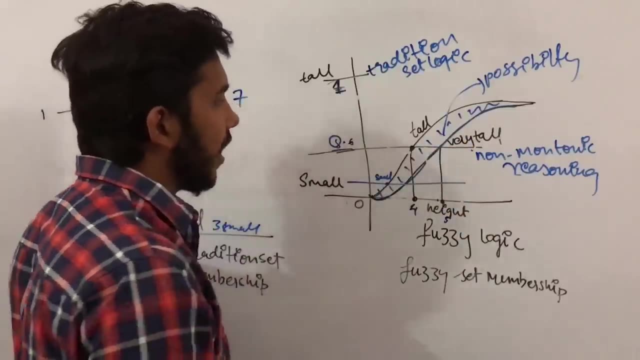 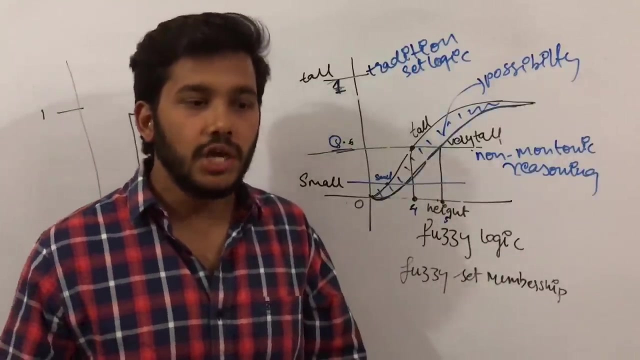 the incomplete information for this value 5 suppose 0.6 corresponds to value 4 and for this it correspond to 5. if we say 4 is tall, then with the non-monotonic reasoning, with the incomplete information, we can make further conclusion that 5 is very tall. 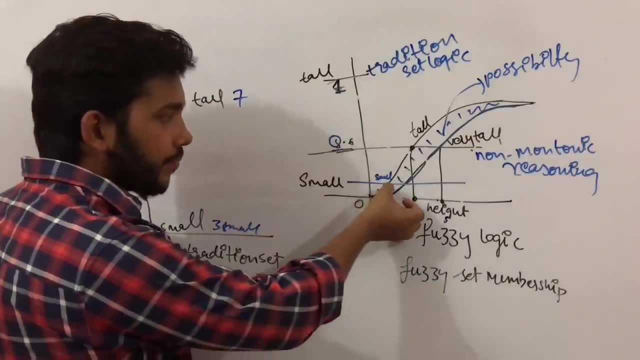 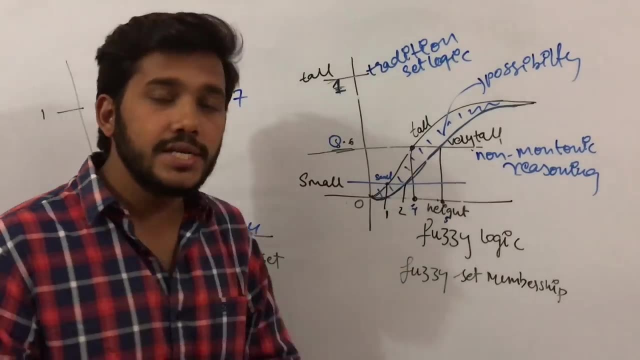 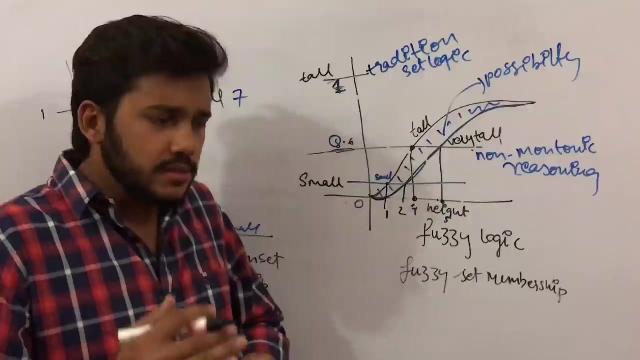 if, if, if, If I said this point, suppose this correspond to 1 and this correspond to 2, then I can say: 1 is small. With this incomplete information, 1 is small. we can say 2 is slightly more than that. 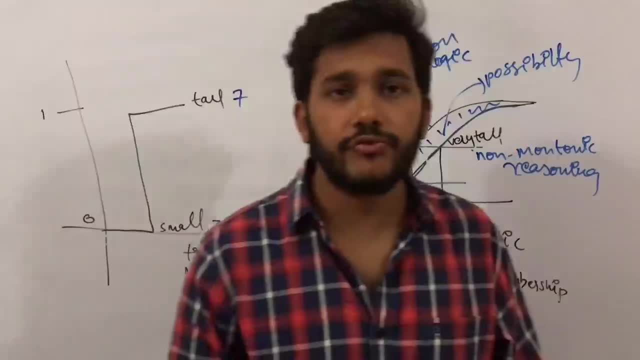 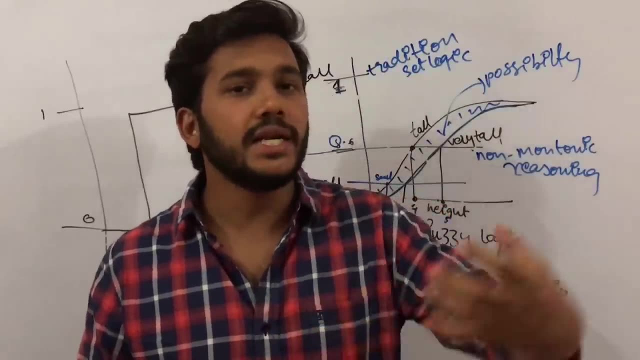 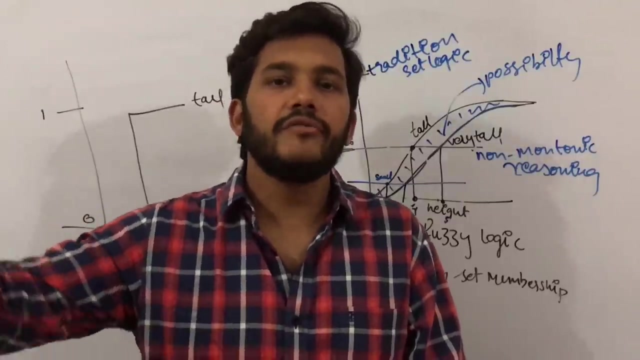 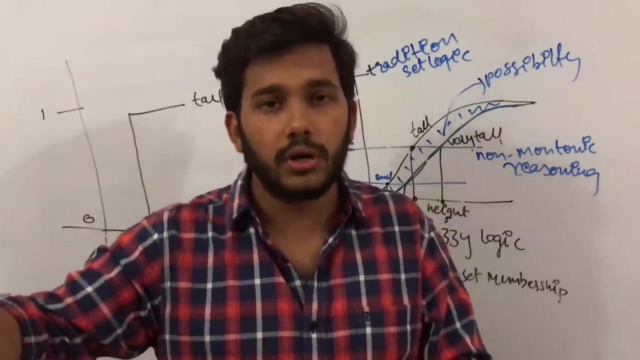 So this was our fuzzy logic. We use fuzzy logic when we want to express the prepositional statement as possibility distribution. When we want to set the different different possibility- like from 3 to 7, we have different different range, like very tall, slightly tall or slightly small, more small or very small. 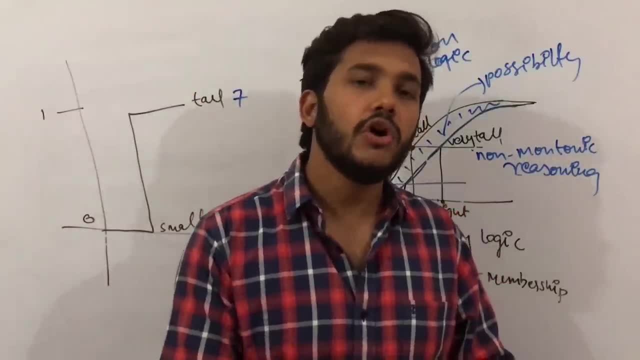 So for this type of statements, we are going to use fuzzy logic. Thank you, Thank you.